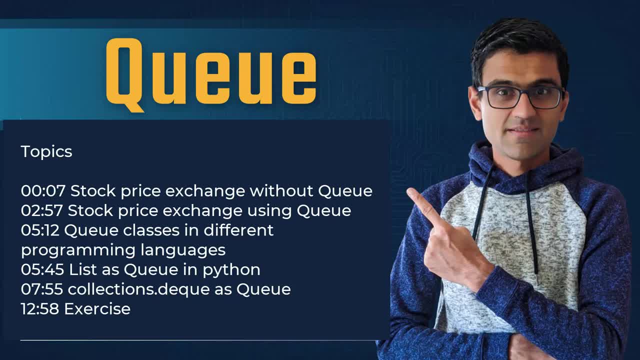 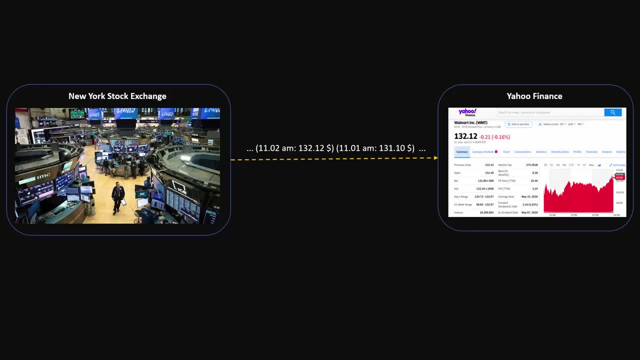 We are going to discuss Q data structure in this tutorial, and here is a list of topics along with their timeline, so if you want to skip ahead, feel free. You might have used portals such as yahoo finance or moneycontrolcom to track down the stock prices. Now the way these portals get stock. 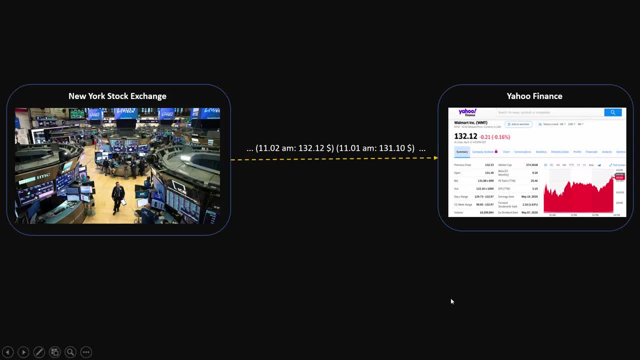 prices is from stock exchanges such as New York stock exchange and if you look at the technical architecture, the engineering things team sitting at new york stock exchange will be supplying the prices. let's say these are the prices for a walmart stock at 11 o'clock, one minute the price. 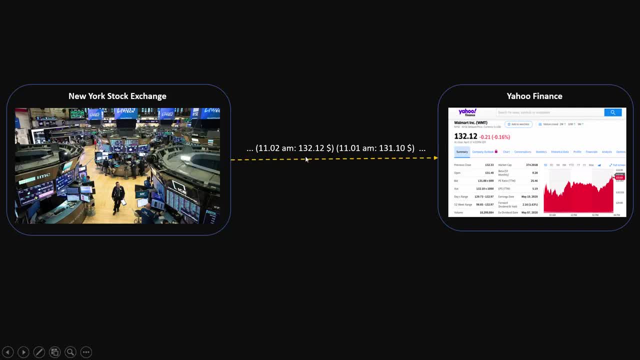 was 131 and then, at two minutes, the price was 132.12.. They supply these prices continuously to a portal like yahoo finance and they will display various charts and information. Now, going to deeper into technical architecture, one way to solve this problem would be the engineering. 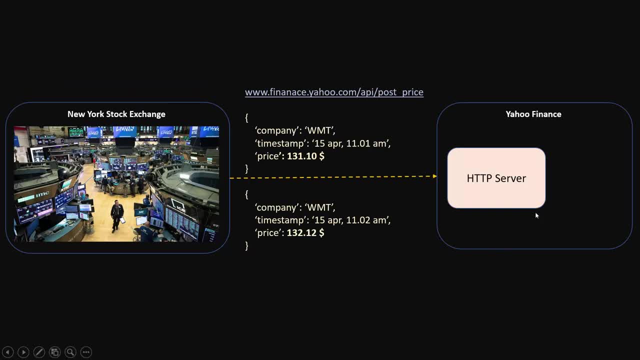 team at yahoo finance will develop an http server which can accept the http post request coming in from new york stock exchange. so the engineering team sitting here in nysc would make http post calls along with these json objects. this could be one architecture and it will work. this way. you can supply the stock prices to the other end. but there are a couple of issues. 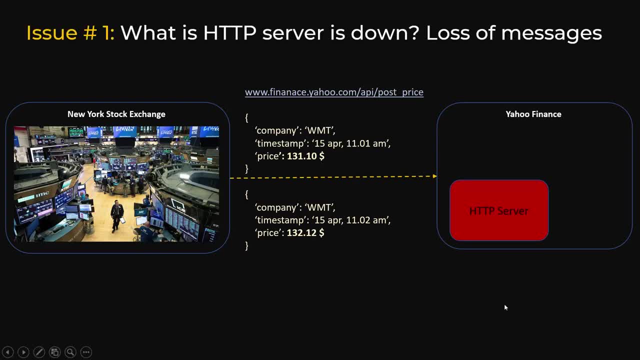 with this architecture. the first problem is: what if the http server is down? in that case, these guys will be making the calls and it will result into loss of messages. so the prices during the time frame that the http server was down would be lost. so all these prices will be lost. 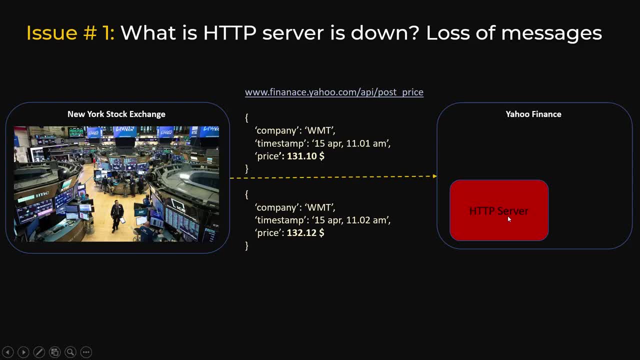 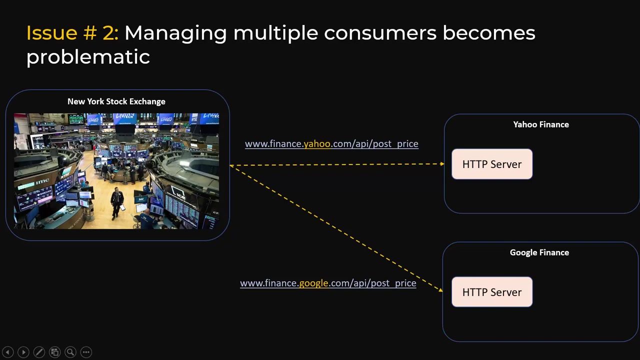 and for yahoo finance, let's say, after five minutes the server comes back up. there is no way to retrieve those old prices because they made these synchronous calls which yahoo finance guys couldn't process because their server was down and now you lost all that information. other issue is tomorrow if google finance wants to receive the same pricing feed. 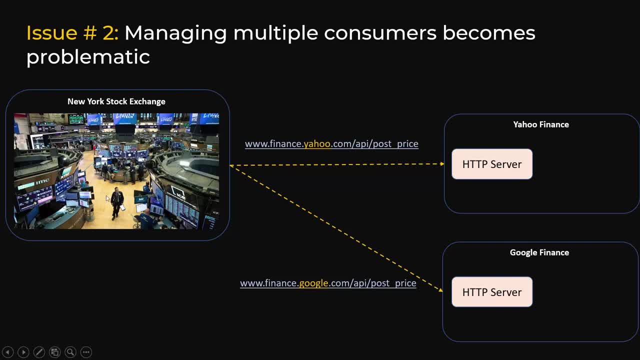 now the engineering team at nysc will have to change their code and use google's url to supply them the prices. this is called tightly coupled architecture and it has a lot of issues, such as: every time you want to onboard a new consumer, you have to make code changes, and if the system is tightly coupled, 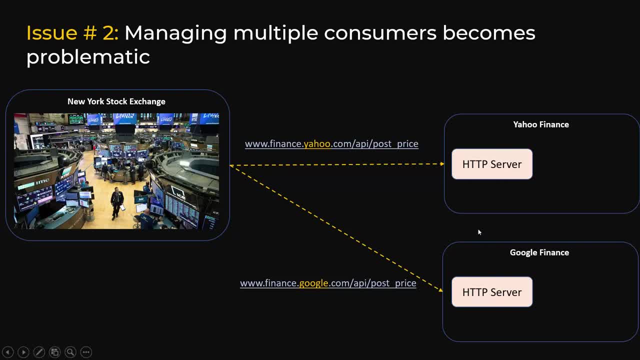 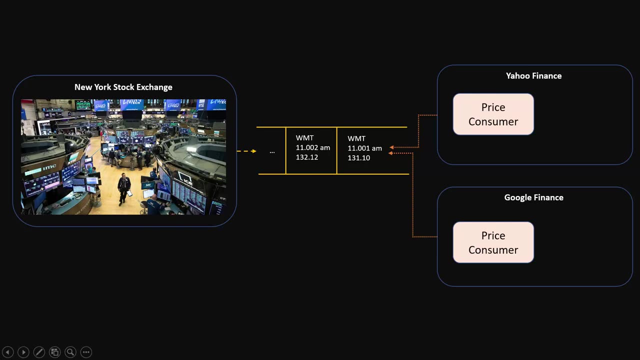 let's say, if there is any change on the consumer side, then producer side will also have to change the code. so it's a nasty infrastructure. there are just a lot of issues. what if you had a memory buffer like this where nysc can just put the prices one by one? so at 11 o'clock, one minute? 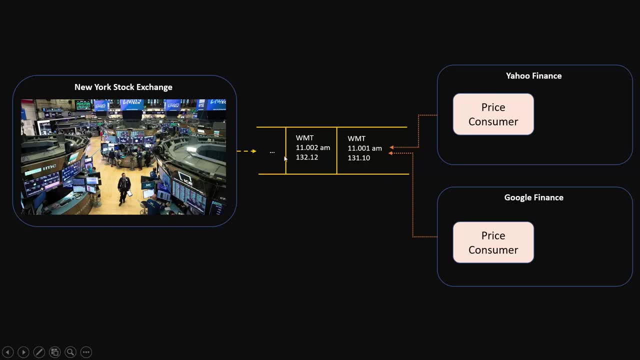 they put this price at two a minute. they put this price and they just keep on pushing these prices and on the other hand side, yahoo finance or google finance guys can make order to receive these prices in the order that they were pushed in. now there are ways where. 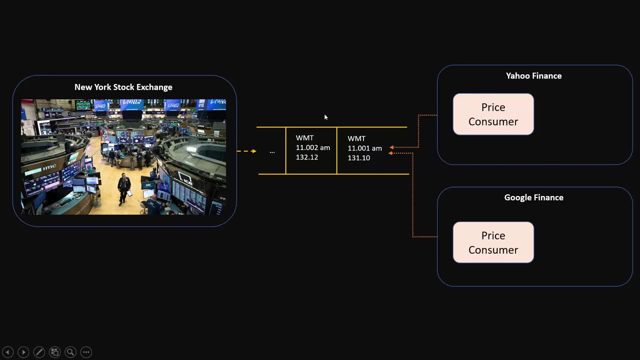 once yahoo finance consumes this particular price, you know their pointer will move here, so that google finance can still consume this. it's not like once yahoo finance consumed this price, google finance cannot consume it. they will have a different pointer, so that will work out. so don't. 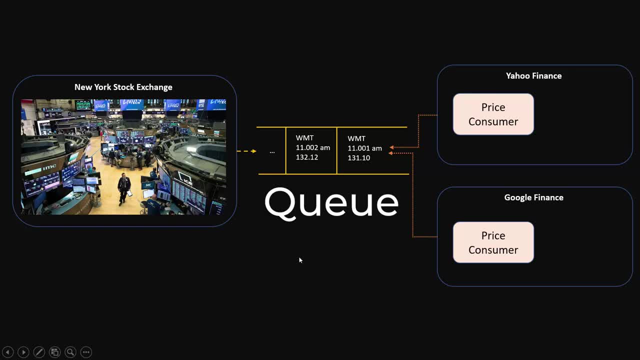 worry about that, uh, but this data structure that we used here is called q, And Q allows you to establish loose coupling. So when there is a loose coupling between these systems tomorrow, let's say, if moneycontrolcom wants to use these prices, NYSC doesn't have to make any change. actually, 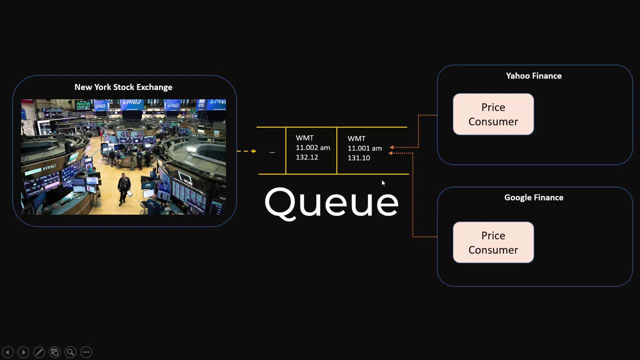 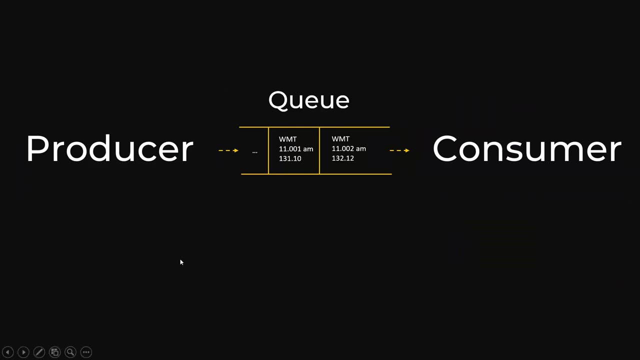 They can just keep on pushing the prices to the same memory buffer and moneycontrol can just consume it. So it's a very flexible infrastructure with minimum amount of issue. This problem is also called producer-consumer problem, where one entity is producing some information and one other entity is consuming the information produced by a producer in a way that they are not tightly coupled. 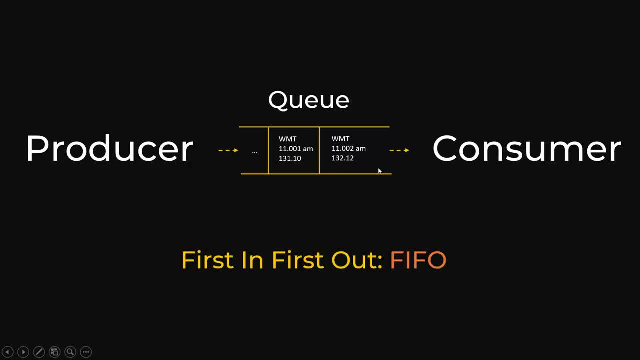 Here, whatever is pushed first in the buffer is consumed first. hence it is called FIFO or first-in-first-out data structure. If you remember from our last video, the stack data structure- it was last-in-first-out versus Q- is first-in-first-out and you have already noticed Q in real life. 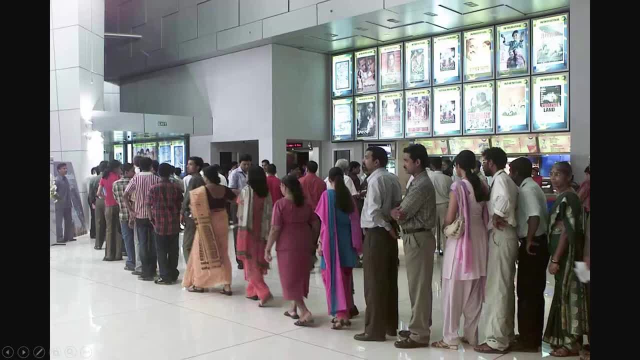 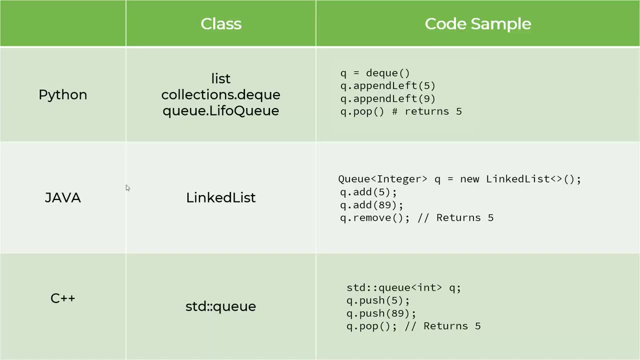 Let's say, if you are at a movie theater buying tickets, whoever is standing first will get the first turn, So it's like first-in-first-out. These are the code snippets in different programming languages for Q, along with their Q classes. For example, Java uses Linkless. 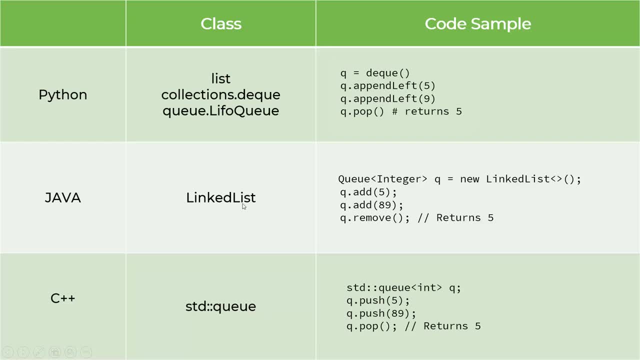 As a Q implementation. So this is not a typo. It actually uses Linkless as an implementation for Q. So Q is an interface which is implemented by Linkless data structure. Here you see like you are adding FI on 89 and when you say remove, you will get FI back. 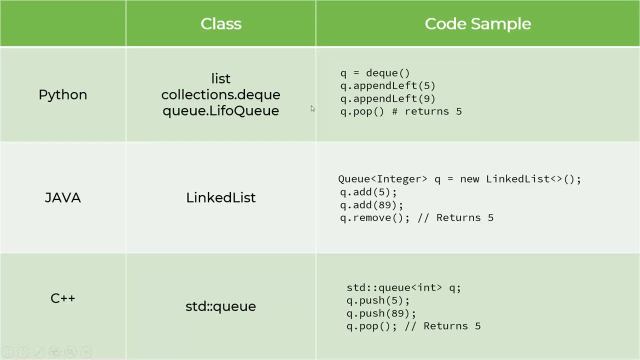 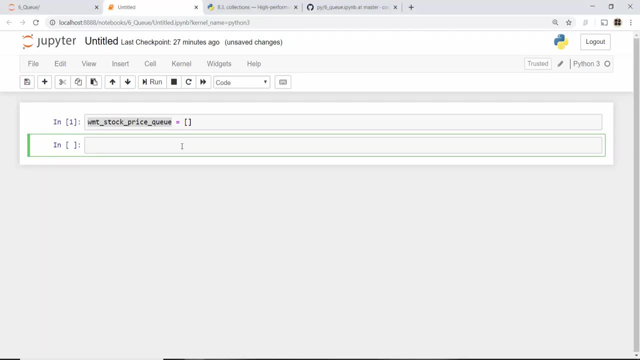 Similarly in Python. you can use one of these three approaches to implement Q. Now we will see how to use Q in Python. You can use list as a Q in Python. Here I have a list. I have created a list called Walmart stock price Q. 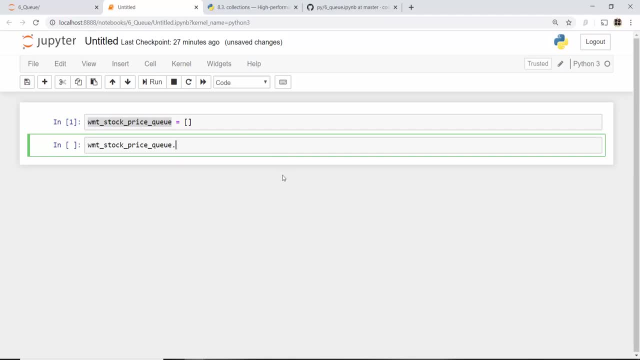 And whenever you want to insert an element in the Q, you can use this insert operation. You are always inserting at the 0th position. So the first price that you had was this And the second price you had was this. let's say: 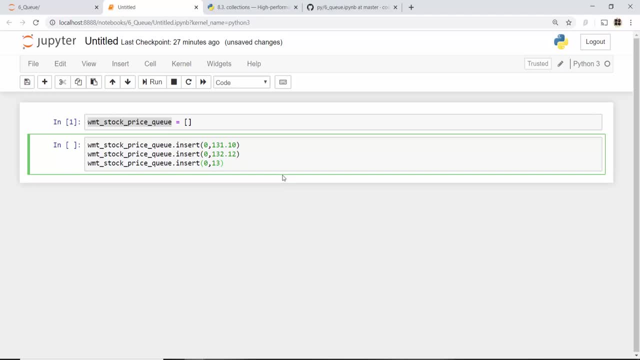 And let me insert one more price called 135.. Every time when I insert a price, I have to insert another price. Every time when I insert an element at the 0th position, the remaining elements get pushed forward. Okay, When you do this and when I look at my Q right now, 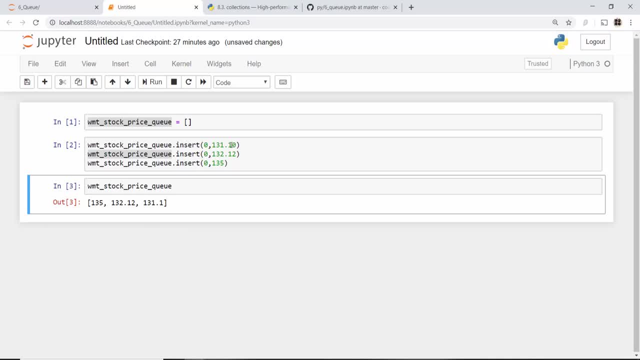 So the Q will look like this. So you see, you inserted 131 first, So 131 is here, then 132, 135.. Now when you do pop, Q is first in first out. data structure Stack is last in first out. 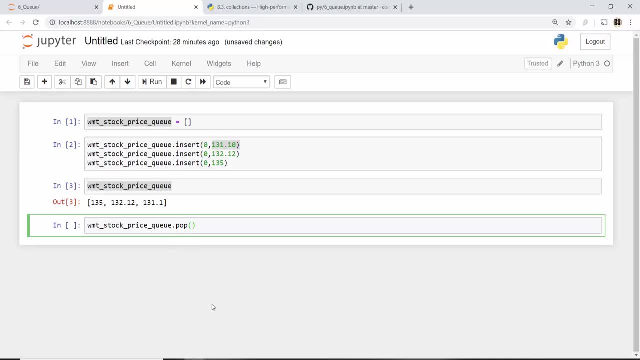 So when I do pop, just tell me, what do you expect to get out of this pop operation. It is first in, first out. So the first thing that was in was 131.10.. When you do pop, see, you got that thing back. 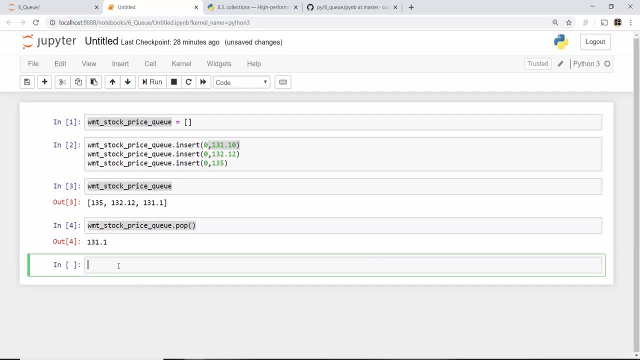 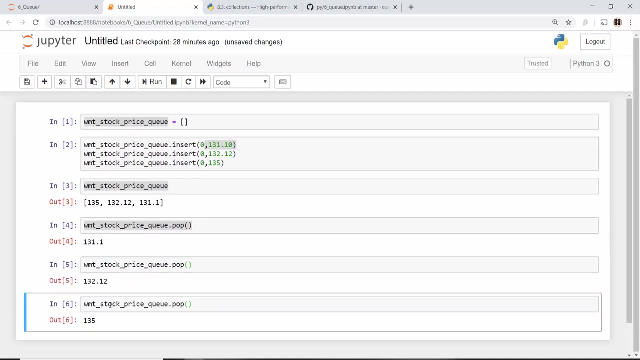 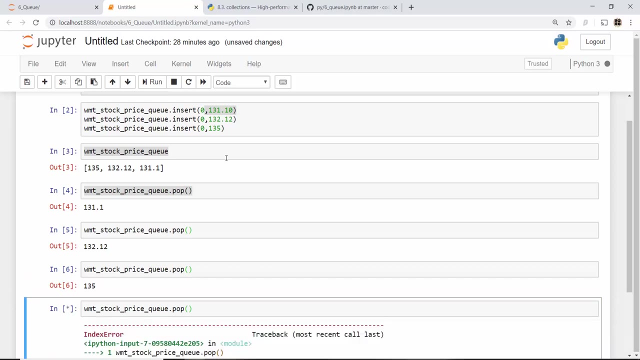 When you do pop again, you will get 132.. 132.12.. Pop again. you got the last element, 135.. Now my Q is empty. So when I do pop again, imagine what's going to happen. Yes, it's going to throw an exception. 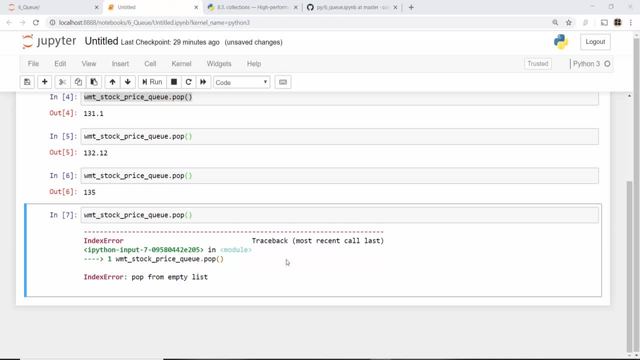 While list can work okay as a Q, it has problems associated with dynamic array. In our past tutorials we have seen what kind of issues you might face when you are using dynamic array, Such as when you're allocating new elements And if it exceeds the capacity, it will have to allocate new memory area. 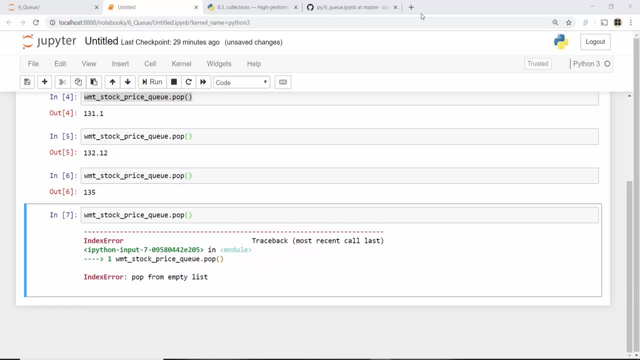 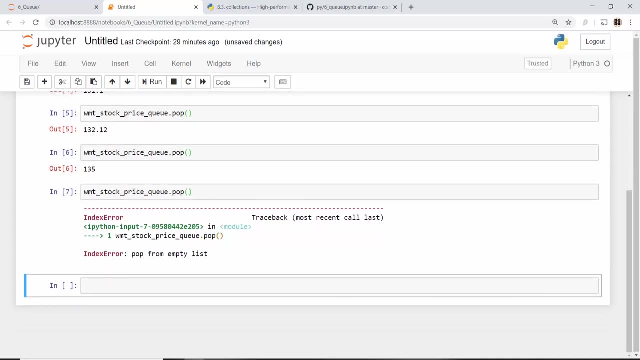 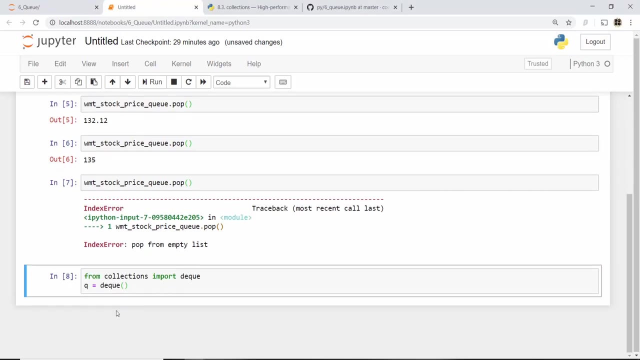 And then it will have to copy all those elements. Okay, So using list is not very much recommended as a Q. You can use other approach, which is using DQ from collections module. Now, in last tutorial we used DQ as a stack. 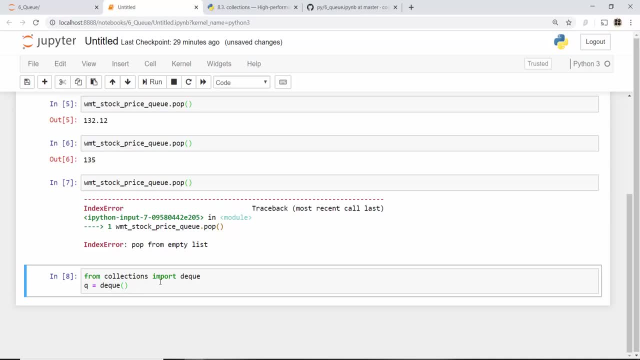 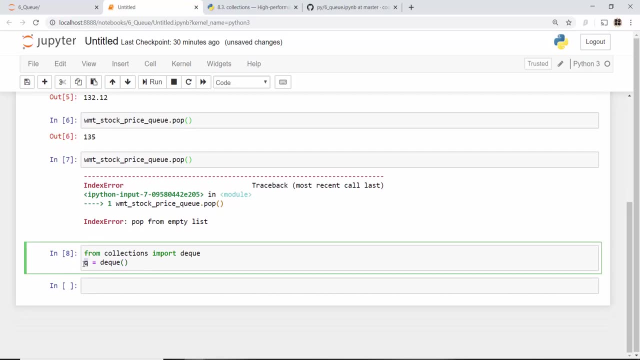 So DQ is double-ended Q. It's very flexible, It works. It can be used as a stack as well as a queue. So here I have created a variable called Q, which is an instance of DQ, And let's see how we can use it as our Q data structure. 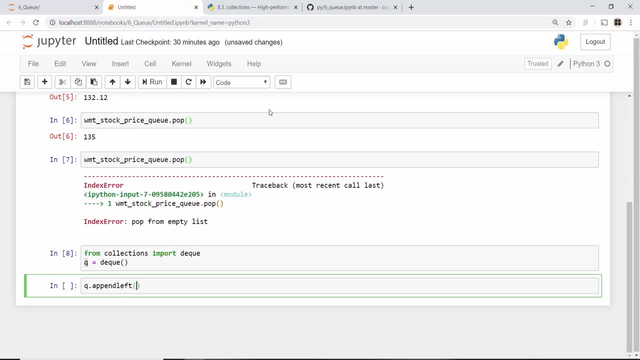 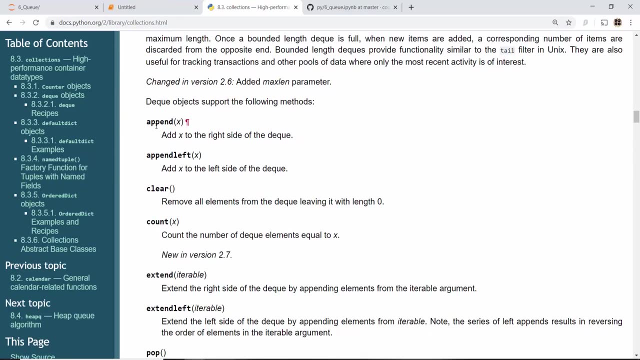 So this has a function called append left. This is the documentation of DQ. If it was stack, we would have used append. We already did that in our last tutorial on stack, But in Q you're always appending at the left-hand side. 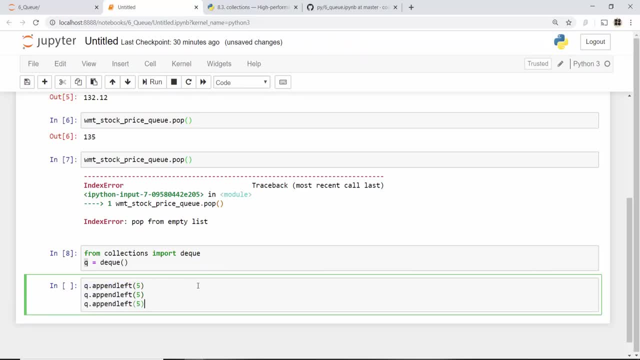 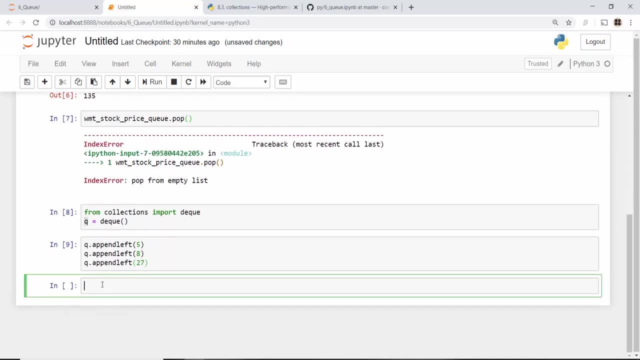 So I'll append bunch of values. Okay, So let me append whatever some random values, And then when I do Q dot pop, tell me what do you expect? Q is first in, first out data structure. So whoever got first in, you know five. 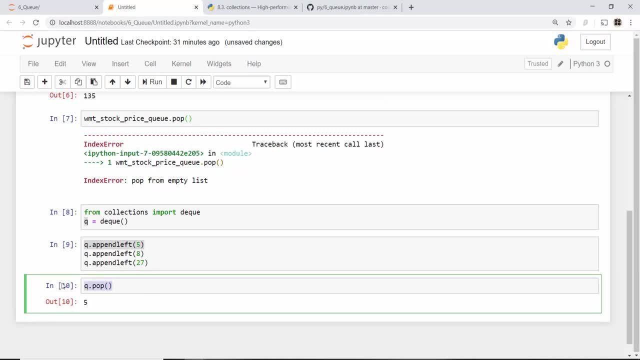 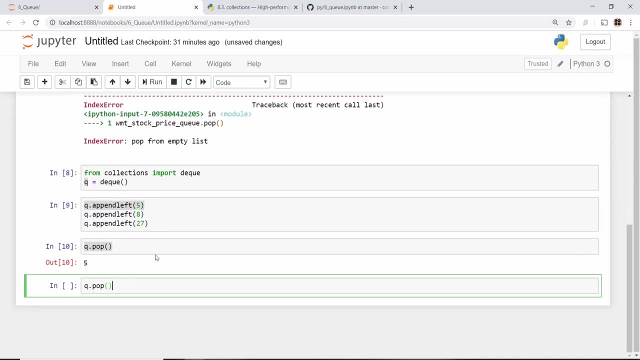 That comes out first, Very obvious, Like if you're standing in a queue to buy a ticket for your train. whoever got into queue first will get his ticket first. right, It's just a simple principle of Q that we use in our day-to-day life. 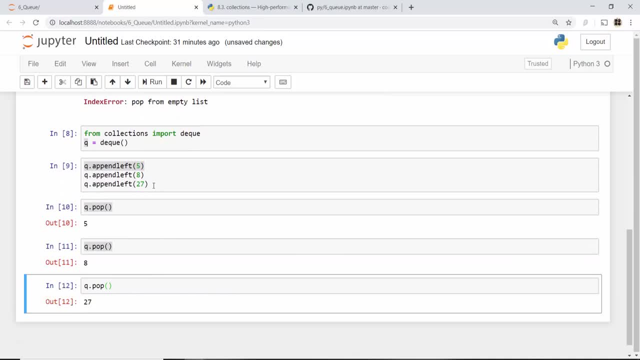 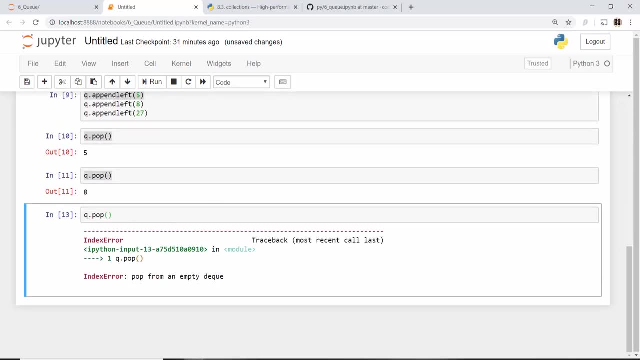 And now you do Q dot pop and you get 27 back. You do Q dot pop one more time And it will throw you an exception. So now let's implement a proper Q class in Python using collection dot DQ, And just to save some time, I'm going to just copy paste the whole class, because the class implementation is pretty simple. 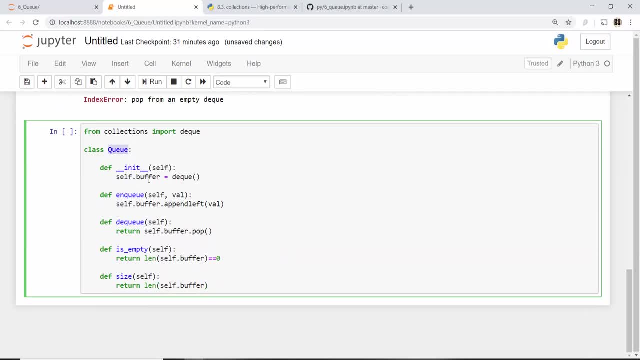 Here I'm creating a class where there is a class object called buffer, which is an instance of DQ. Q will typically have NQ and DQ methods. NQ is placing an element in the queue. It's like you are standing in the queue to buy your movie ticket. 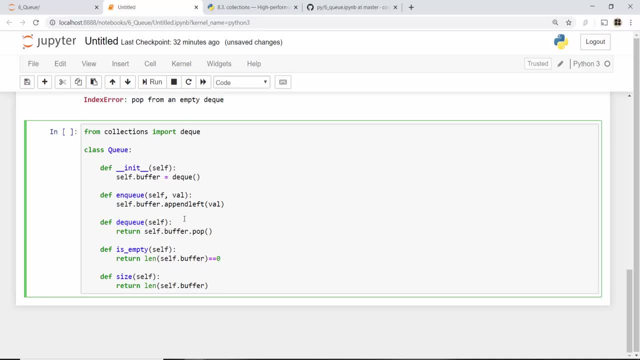 And DQ means you bought your ticket. So now you are out of the queue And these are helper methods, whether the queue is empty or not. And what is the size? So if you look at this class, pretty straightforward, very, very simple class. 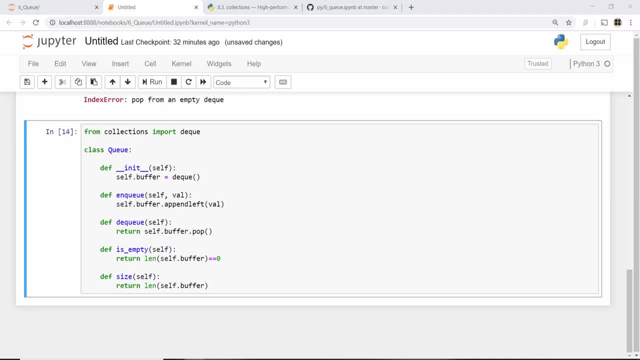 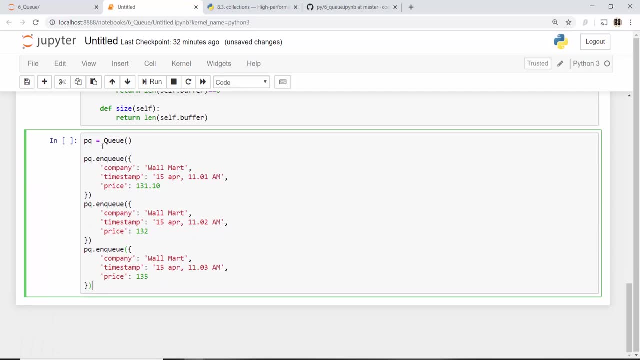 Okay, And we can use now our Walmart stock exchange Price example to put a couple of elements. So here I created a queue using this queue object And then I have inserted a couple of dictionary elements. which represents Walmart stock price? Okay, 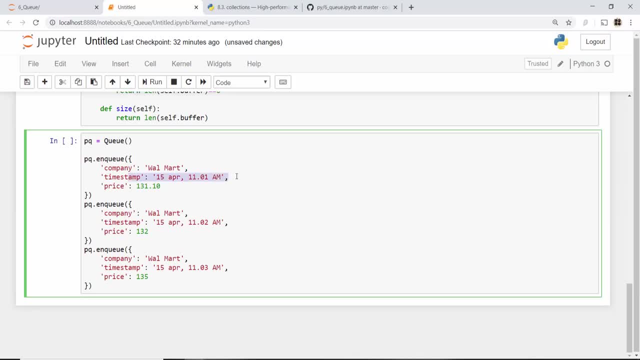 So I have a typo. I'm going to remove that And these are the stock prices. So at 11 o'clock one minute, 11 o'clock, two minutes, three minutes, different prices, And I use NQ to put all those elements in the queue. 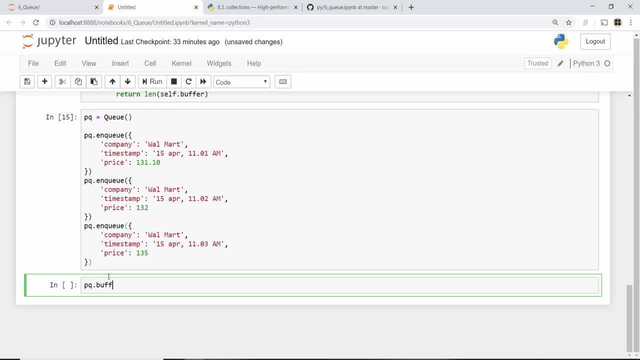 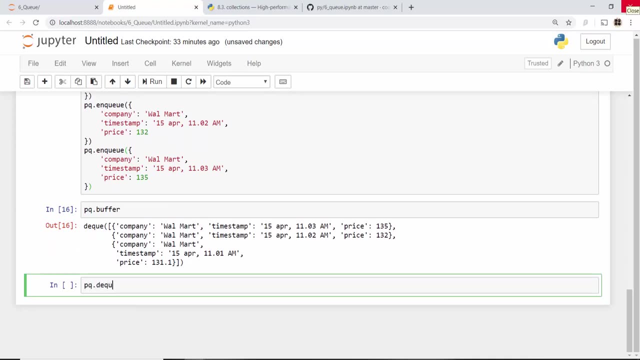 When I print PQ dot buffer, it will show me all these elements, Okay, One by one. And when I do PQ dot DQ. So just think about this as your Yahoo finance code. So the engineering team on the Yahoo finance side, they will use DQ. 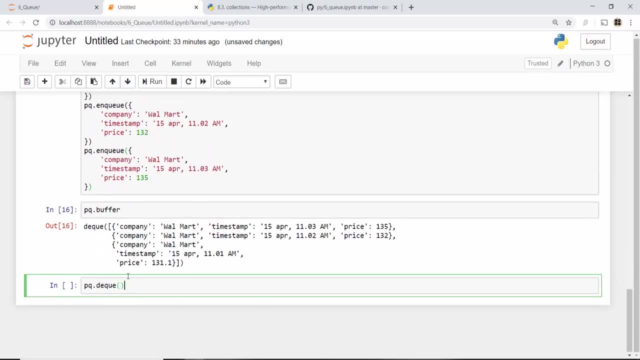 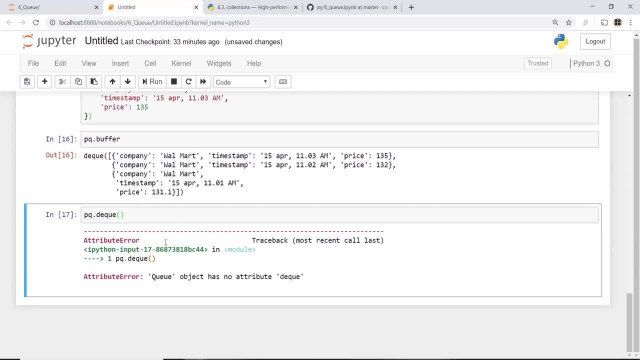 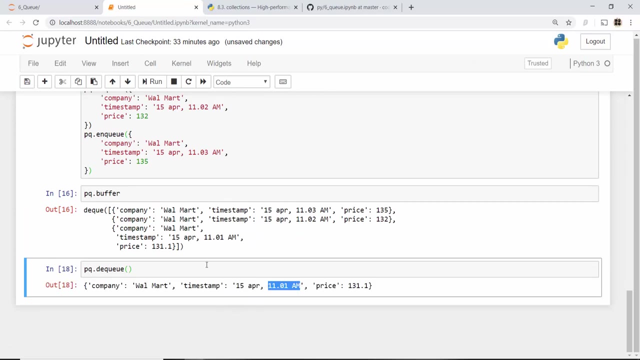 Whereas on New York stock exchange side they will NQ. They will NQ all the prices. Okay, So at Yahoo finance, when I say DQ, D-Q-U-E-U-E- again a typo- I will get the first price at 11 o'clock and one minute. 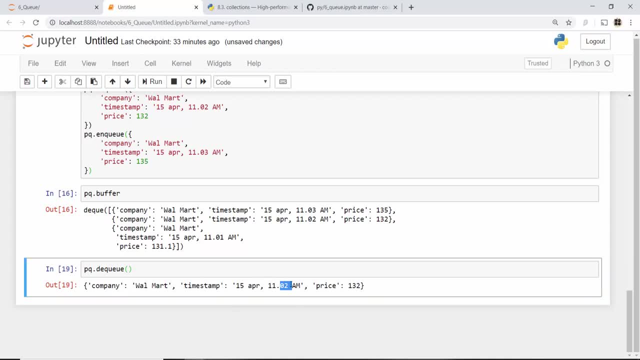 When I run this same code again- see 11 o'clock and two. same code, again 11 o'clock three. So this way I can keep on accessing these elements one by one. I just quickly show you the size method. So I ran this again. 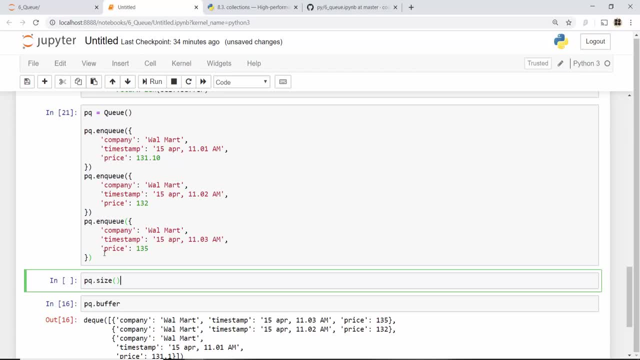 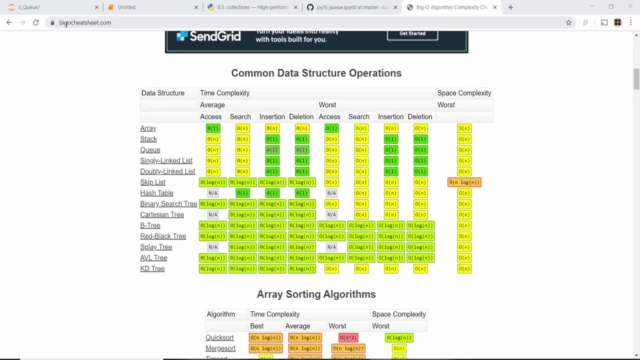 And if you do PQ dot size, it prints the size as three. So that's all I had for coding part. There is a website called bigocheatsheetcom which will show you the big O complexities for different data structures. So here in the queue, data structure, average access and search complexity is order of N. 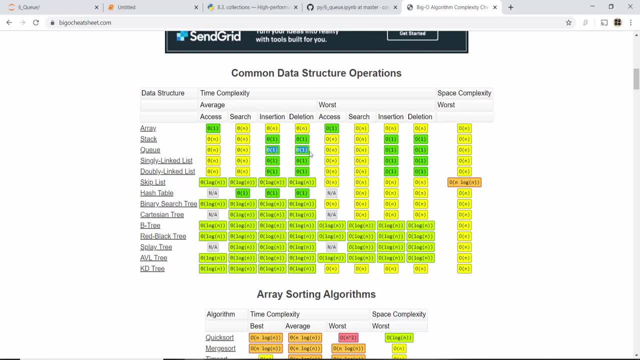 Whereas insertion and deletion is order of one, And these are the worst case complexities, So you can refer to that. I'm going to create more tutorials where I will be comparing different data structures for different type of problems And we'll be doing in-depth big O analysis at that point. 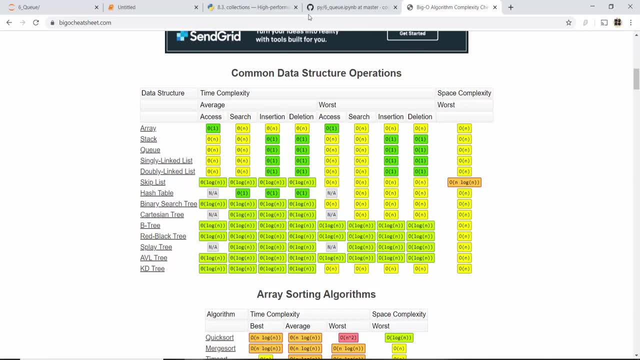 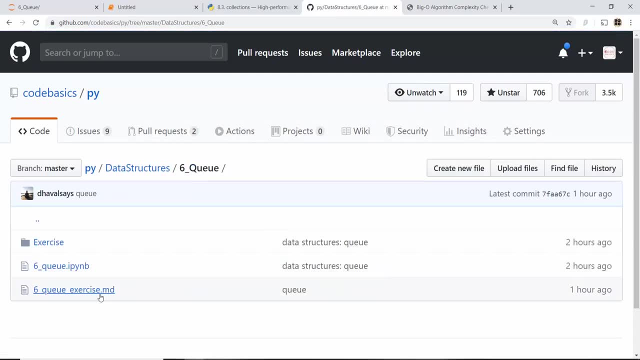 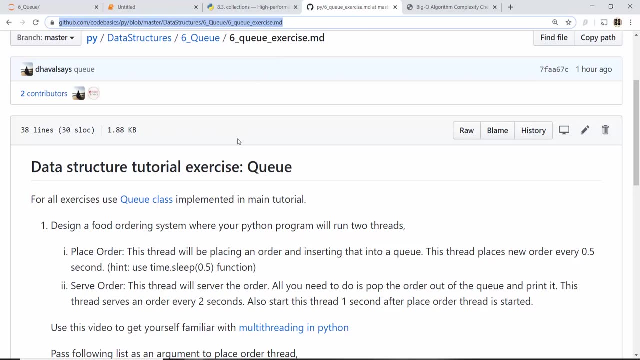 Now moving to the most interesting part of this tutorial, which is an exercise. Yes, I have an exercise for you all And let me open that This GitHub MD page. I'm going to provide a link of this in video description so you can refer to the exercise. 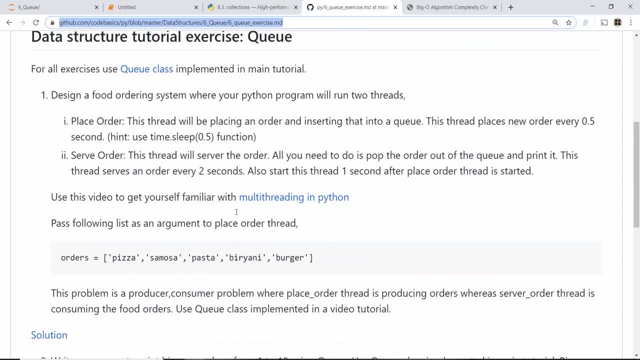 We have two exercise for this tutorial. You can just read through the description. I have provided some important links here, So let me repeat the same thing again and again. I know I'm becoming very boring. just by watching the tutorial You are not going to learn any coding.